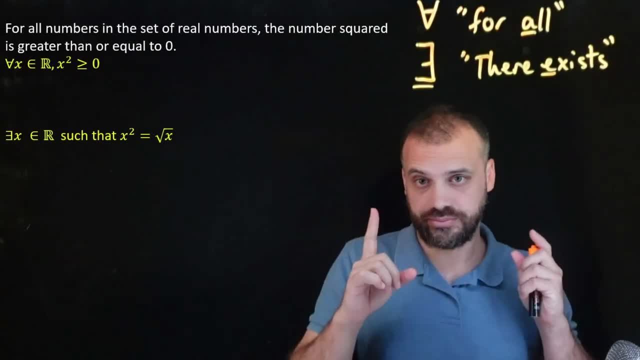 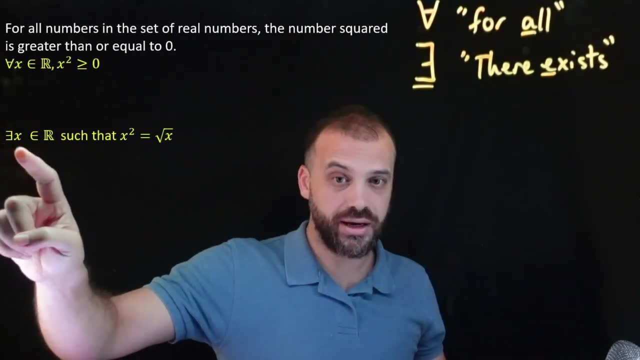 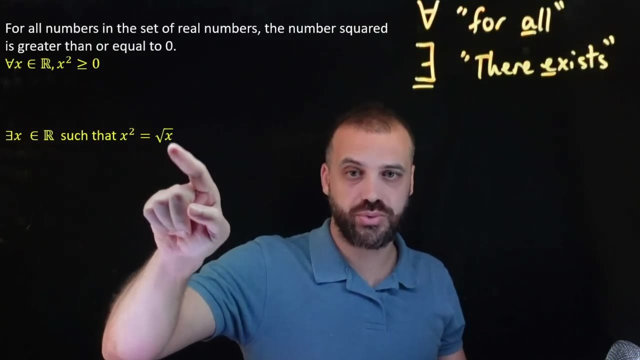 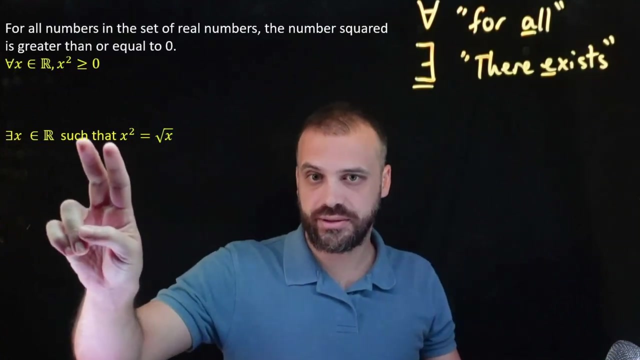 another sentence. Read it, Pause it, Think about it. I'm going to read it now. There exists a number x in the set of real numbers, such that x squared is equal to the square root of x. So there is some number that that is true. for Now I will say: some people believe you probably. 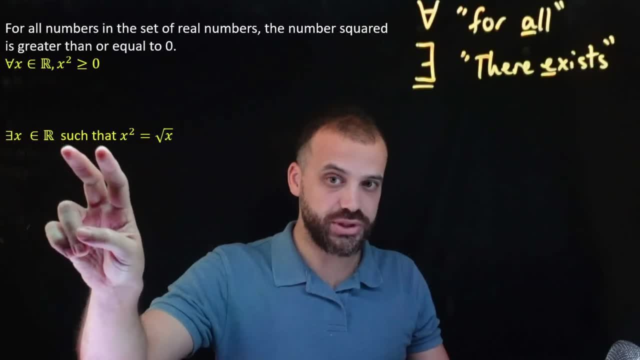 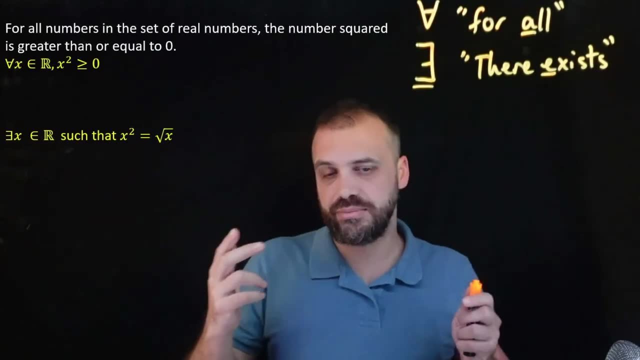 don't need that such that there You could probably just say: there exists a number in the set of real numbers: x squared is equal to root x. but let's keep the such that. there We've got language, We're trying to communicate. It's a bit ambiguous as to whether you should put it there or. 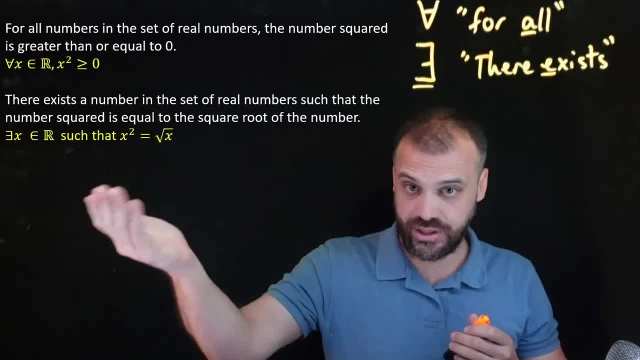 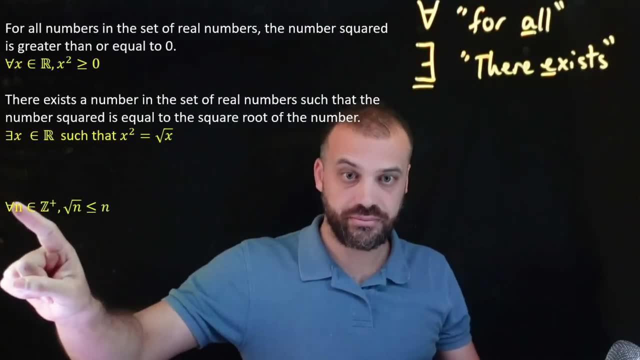 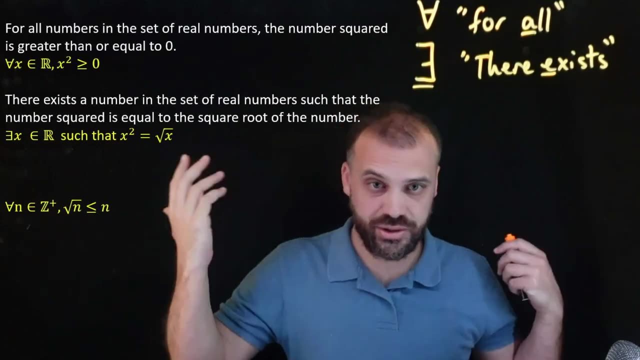 not All right. so that's what that says. Another one: All right. what does this say? Pause it, Try it For all numbers now. I've been using x's so far, but we can use n's, p's, q's, doesn't matter. 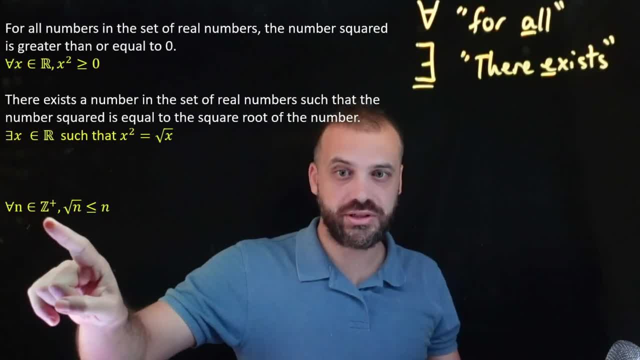 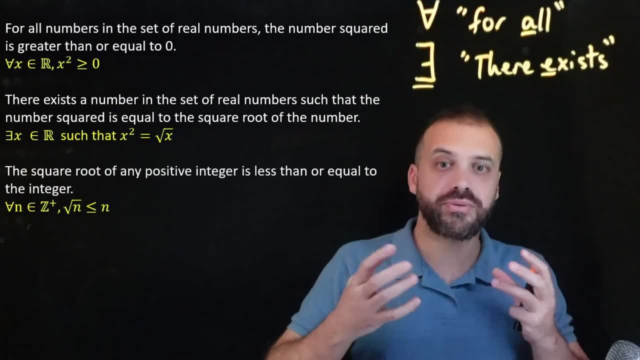 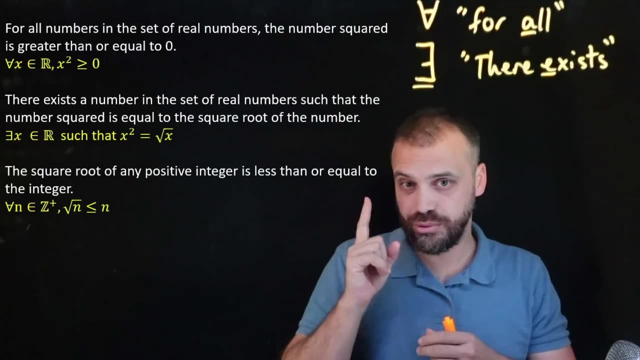 For all numbers in the set of positive integers, the square root of n is less than or equal to zero. All right, so what's most important to me here is that you can read these mathematical sentences. Writing them you might find that trickier, but reading them, that's the important part. 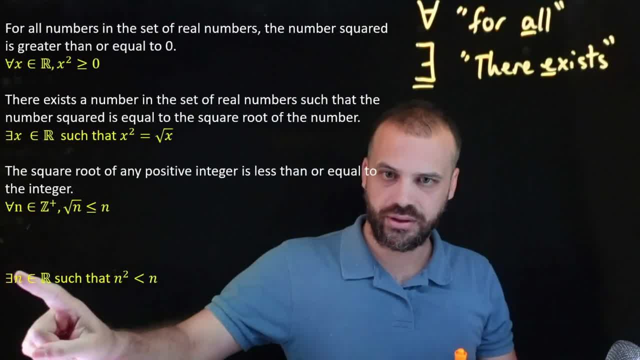 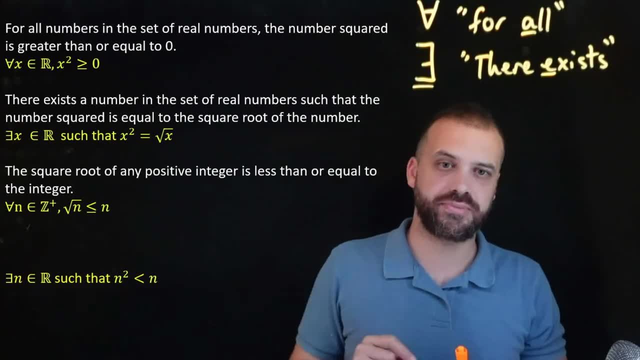 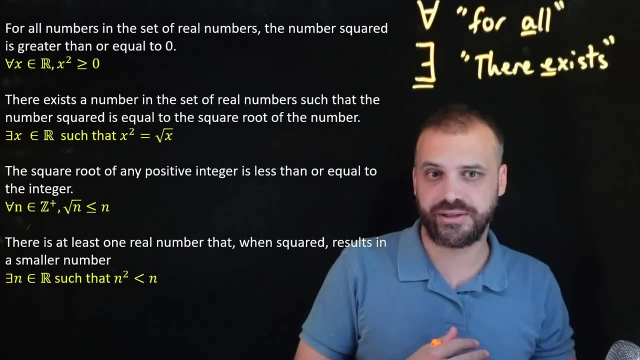 All right, what else have we got? There exists a number in the set of real numbers such that n squared is less than n. Again, we're using that such that, there for clarity, You don't need it. Okay, next up. This is the last one. 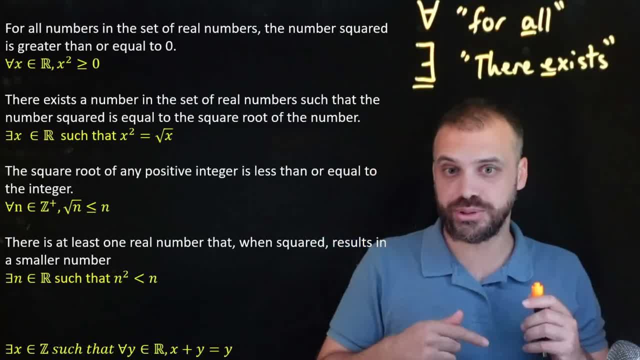 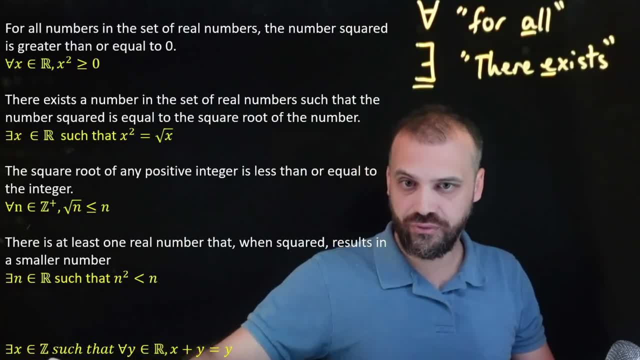 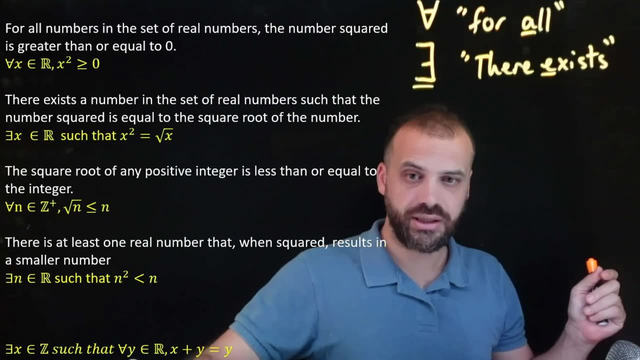 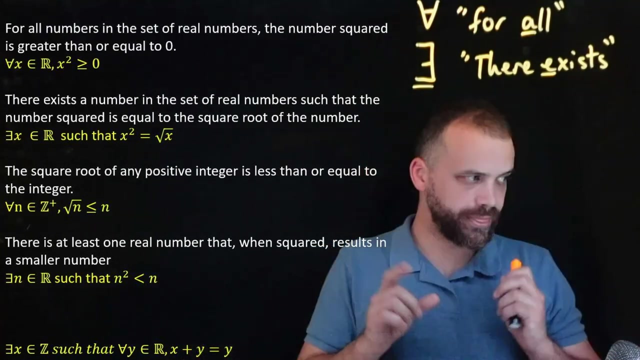 Okay, there's a lot going on here, So let's read through it slowly. There exists a number in the set of integers such that all a different number in the set of real numbers, x plus y, equals y. All right, so there exists some integer such that it doesn't matter what number you add to it. 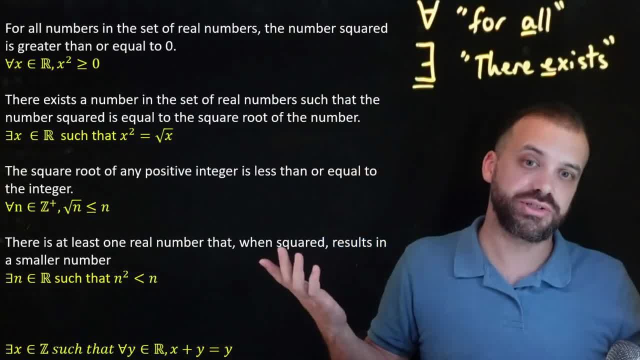 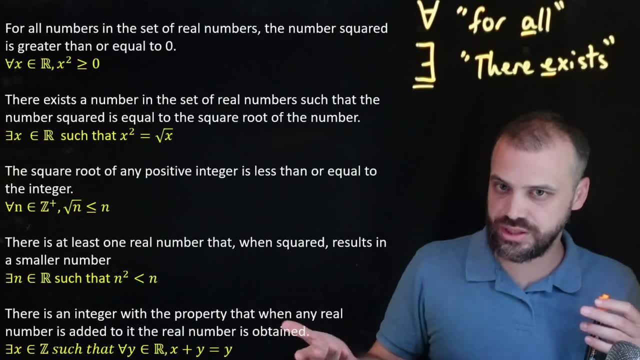 you're going to get the number that you added to it And that integer is zero. Zero plus any number makes the number that you started with All right. so it's a bit of a doozy there. You can see we've got both of our symbols.